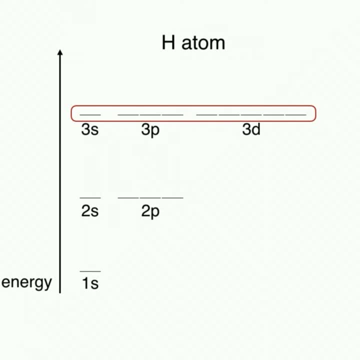 are in line with each other. This means they all contain the same amount of energy. Let's now see an energy level diagram for a multi-electron atom. We can see that all orbitals within the same n do not have the same energy. 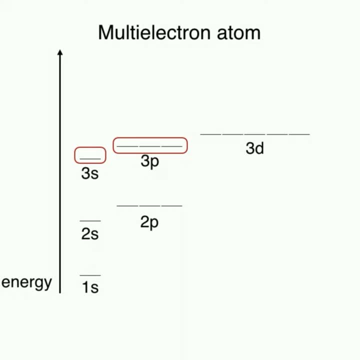 For example, the 3s orbital has less energy than the 3p orbitals, which have less energy than 3d orbitals. The same holds true for 2s orbitals and 2p orbitals. This is due to the electron-electron repulsions. 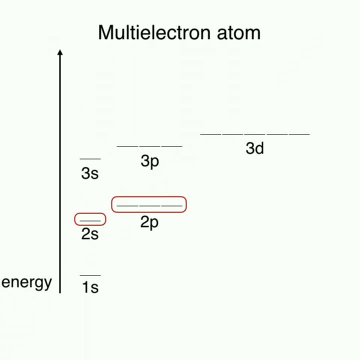 found in multi-electron atoms. Another important note is that the energy of each given orbital is lower in this diagram than in the hydrogen diagram. For example, a 2p orbital in a multi-electron atom has a lower energy than a 2p electron. 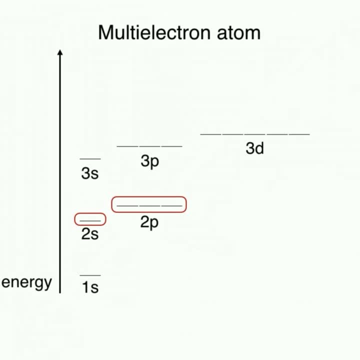 atom. For example, a 2p orbital in a multi-electron atom has a lower energy than a 2p electron in a hydrogen atom. This is because the greater the number of electrons an atom has, the greater the attraction between the nucleus and the electrons. 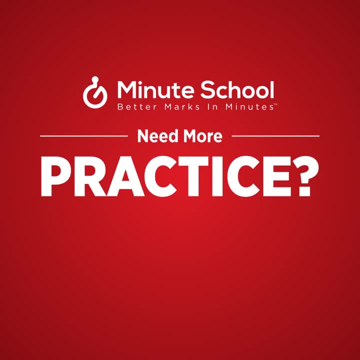 This greater attraction causes the atom to contract and decrease in energy. 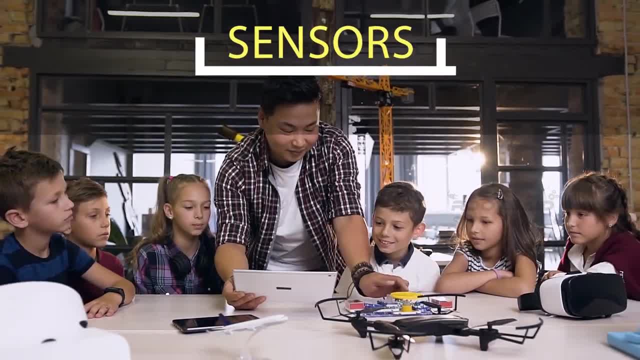 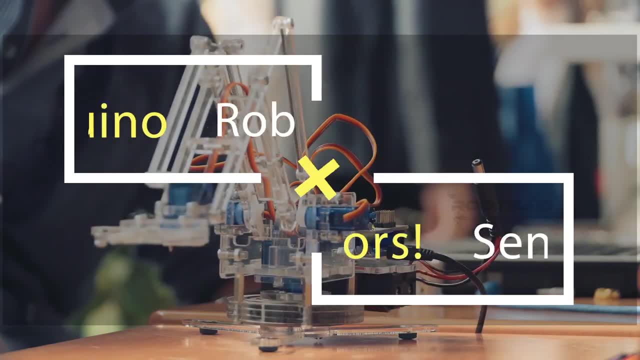 In this video of Robotics for Beginners series, I will explain everything you need to know about sensors, different types of sensors, connecting sensors to Arduino and its application in DIY hobby projects- for you to get started with your own robot. Like the previous video, I will try. 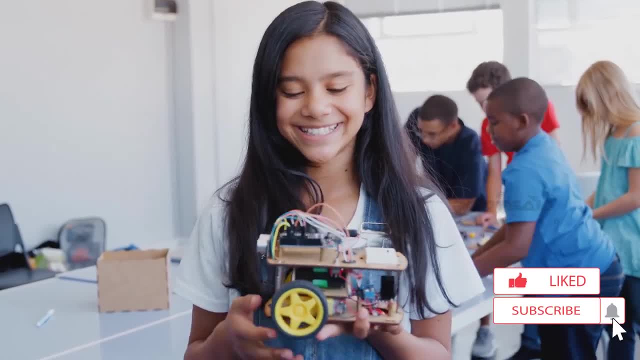 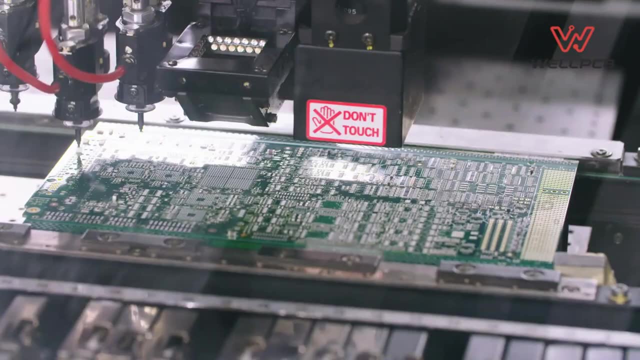 to make this video as interesting and simple as possible, so that everyone can understand everything easily in a fun way. Before going further, let me introduce you to the sponsor of this video: WellPCB, If you want quality PCBs for a low price for your hobby projects.